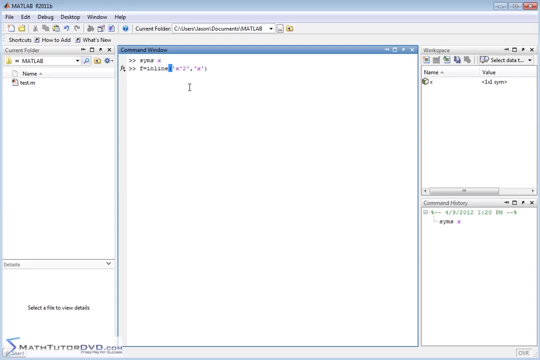 to x squared and the independent variable is x, right? So the first step: we've defined x to be a generic symbol, because all of these calculus things are going to be dealing with symbolic math. and then we calculate or we define this function: f of x is equal to x squared. 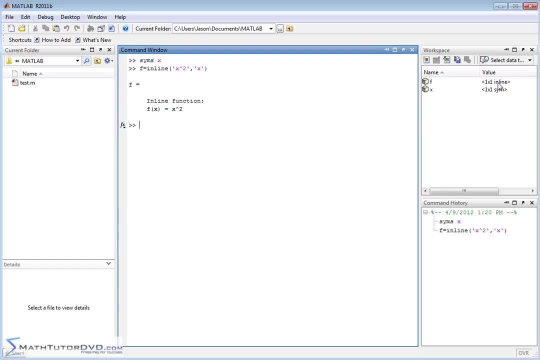 So over here in the workspace we have x, which is a symbol, and f, which is an inline guy, which is MATLAB. speak for it's a function, All right, so we have this here Now. this function behaves just like any other function we've defined. 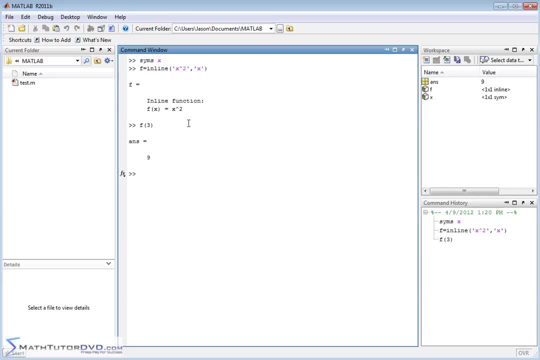 You know, if you plug in a number, you get a number back right. So that was what we covered in the last section. Now what we want to do is calculate the derivative, So the let me go and clear the screen to give us a nice clean slate. 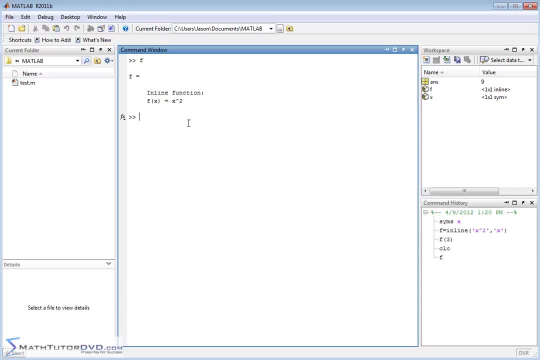 Our function, f, is defined as it is on the screen now, and now we want to calculate the derivative. So the function that does that in MATLAB is d, i, f, f, And what you need to do is tell it what function you're trying to take the derivative of, in this case, f of x. 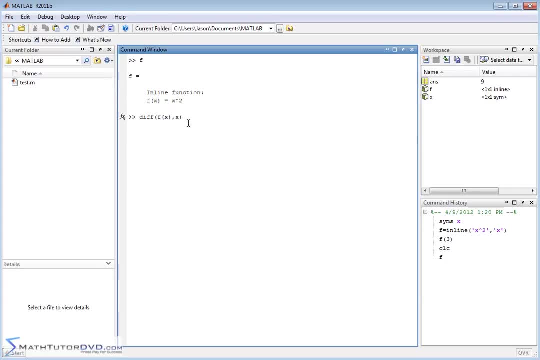 And you also have to tell it what variable you're trying to take the derivative with respect to. So this is easy because it's a simple function. it's going to be, you know, f of x and you're taking the derivative with respect to x. 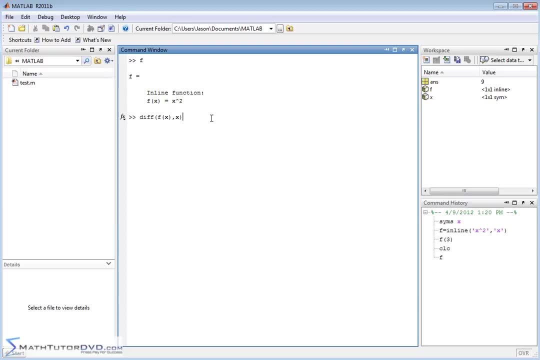 But you still have to specify what variable you're taking the derivative with respect to. All right. so we hit enter and MATLAB calculates that symbolically and it gets an answer of 2x, Which I chose a very simple example here because I want you to realize that you know it's doing what you think it should do. 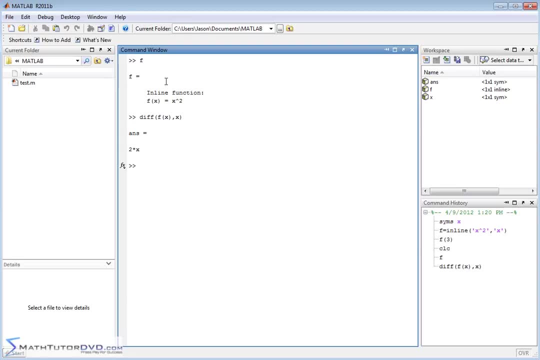 So again, the first step, when you're doing calculus, Define your independent variable as a symbol, like we did here. Then define your function, then you can pass the derivative off to it. All right, so we can continue to play this game. we can. we can define more and more complicated functions, or we can change variables. 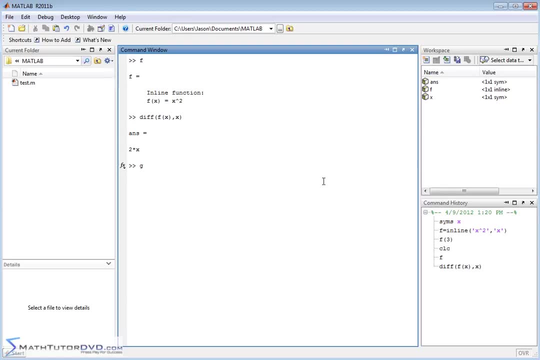 Let's do that for a second. Let's say we have another function, we'll call it g and we'll set that equal to something else here. Let's say g of x, let's call it So. let's say it's sine of x over. 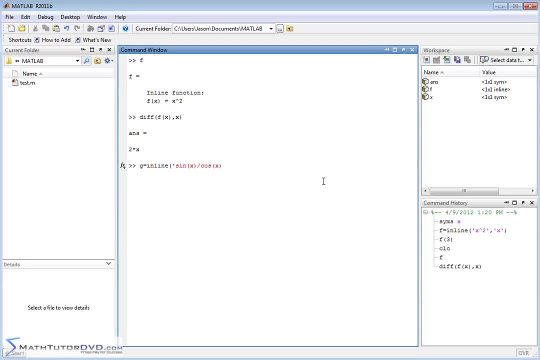 Cosine of x, right sine of x over cosine of x, and we want to obviously have the independent variable as x. So we're saying g of x is equal to sine over cosine. So we have this nice function. of course, g behaves just like any other function. you pass a number to it. 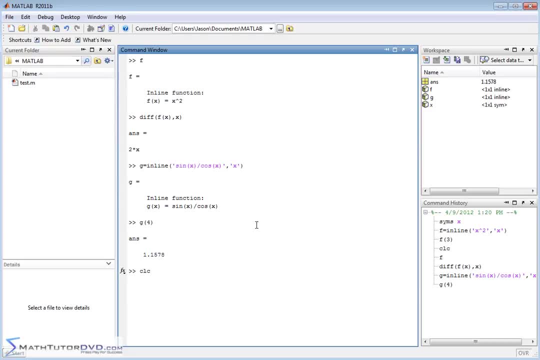 It takes the sine over the cosine and you get your answer back. So we'll clear. the screen. g of x is up on the screen and now we want to take the derivative of this function. So we say d, i, f, f, G of x and we want to take this derivative with respect to x. 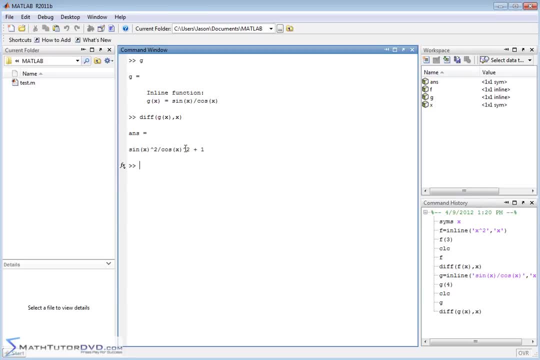 And so it goes and calculates an exact answer: sine squared of x over cosine squared of x plus one. And if you want to make it look a little pretty, you can just take the last answer and dump it in the pretty function and you can sort of, you know, visualize it a little bit better. 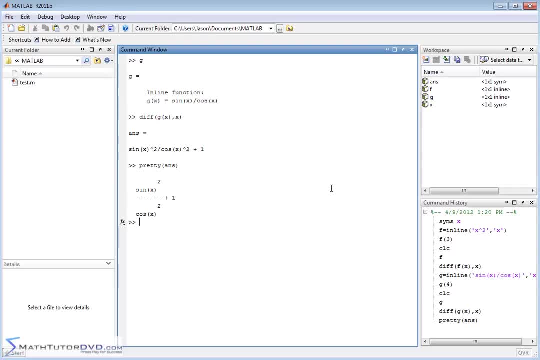 Sine squared over cosine squared plus one, That's the exact derivative. So that is sort of the essentials of how to calculate a derivative in MATLAB. You have to Define the function. You must define the independent variable as a symbol. So let me give you just one final example. 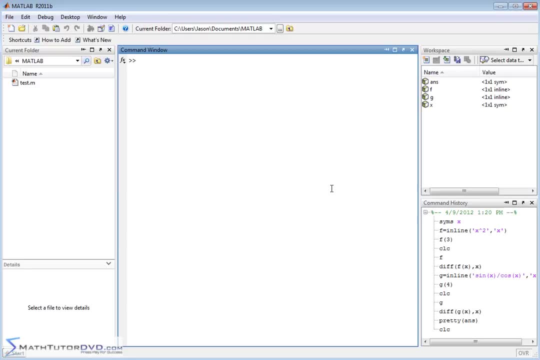 Let's say, our independent variable is: you know u, So you have to do sims u And in fact let's not do it first, Let's just show you what happens. Let's create a function, we'll call it json And we'll do inline of what do we want to do with this function? 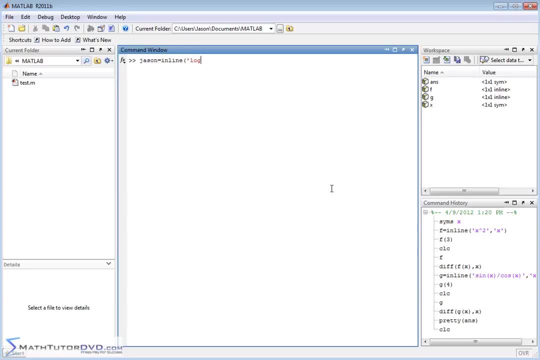 Let's make it a function of u, And this function will just say: it's a log of u plus u. Right, And we'll do u like this. Okay, So we did not. we did not define u to be a symbol, but that's okay, because when we define, 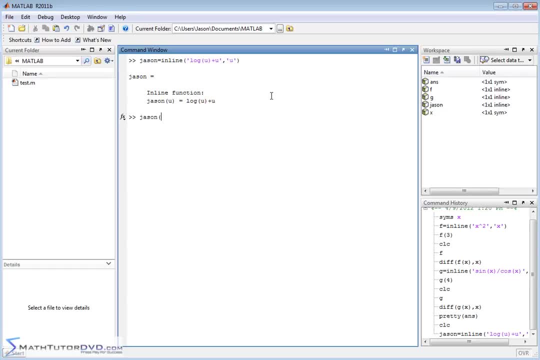 our function. the function is defined fine and the function behaves fine. If I put a number in there, it works just fine. So, defining the function, you don't have to make u a symbol in order to do that. You just define the function and MATLAB kind of treats this as almost like a dummy variable. 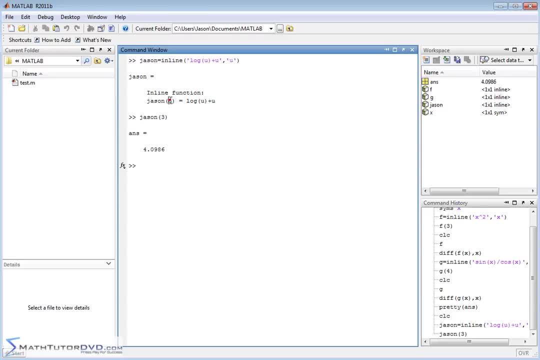 Notice there's no u over here anywhere. That's because when you define this function, MATLAB just treats it as a dummy variable, So you can't just do that. It knows it's just a temporary storage to calculate the function, So it doesn't generate a workspace variable for that.